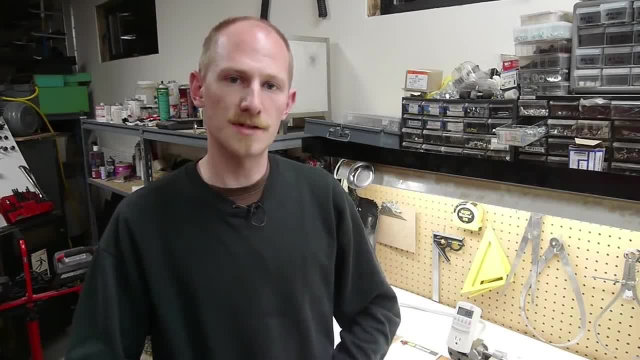 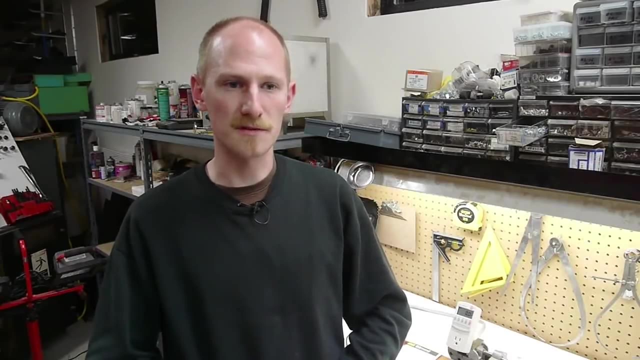 Hey everyone. I thought I'd talk a little bit today about electrical impedance. This is a topic that confuses a lot of people, probably because it's taught sort of backwards, in my opinion, where a lot of people you know spend all their time on the heavy duty math involved and then kind of end with a practical circuit. But I like to go the other way and start with a practical circuit And then, as we move along, uncover the topics as they become relevant. So let me show you what I have set up today. 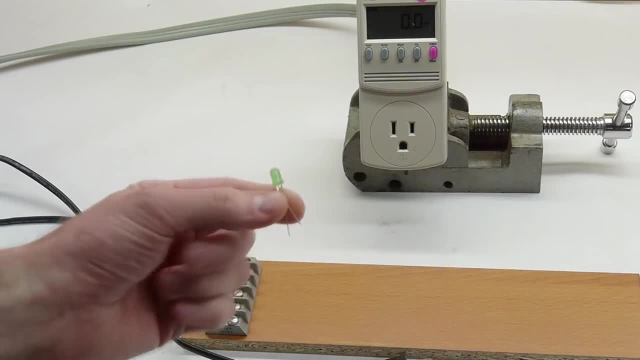 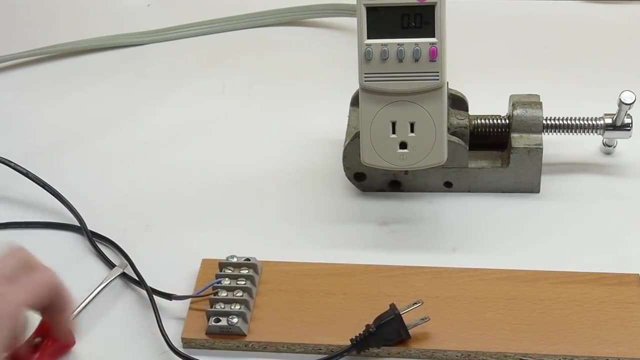 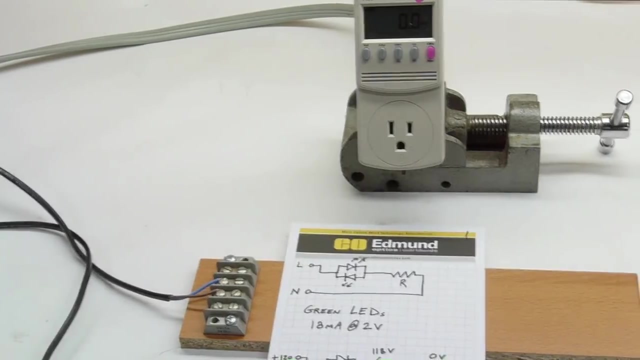 Our task for today is to build a circuit that can power just a standard, cheapo, plain LED directly from the AC mains, while using as few components as possible, and to do it in a relatively energy efficient manner. So to start, we may come up with a circuit that looks something like this, where the LEDs are set up back to back. 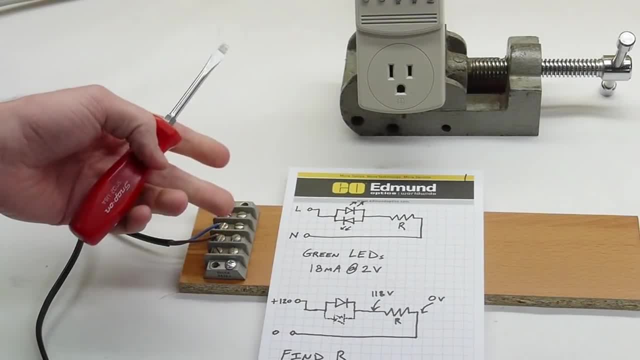 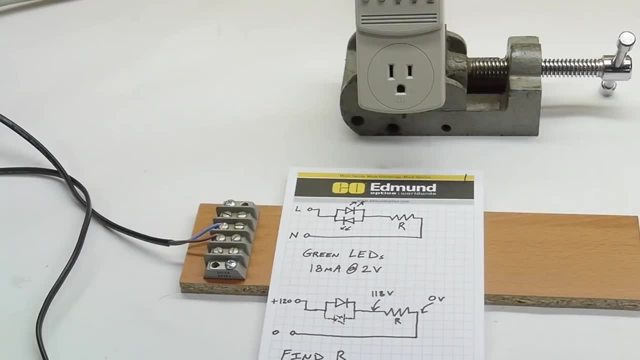 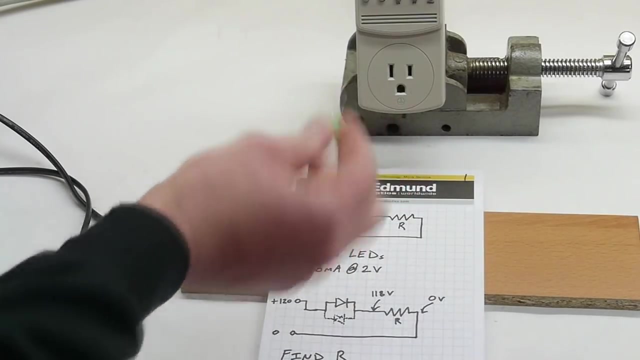 So that as the AC power switches direction, one of the LEDs will light up. So one will be on for both halves of the cycle. But obviously we can't connect the LED right up to house current because the voltage is so high that there would be way too much current flowing. So if you just took an LED- don't do this, by the way- and just put it right into the outlet, it would probably explode in a violent pop because the amount of current would be measured in you know hundreds or thousands of amps or something. 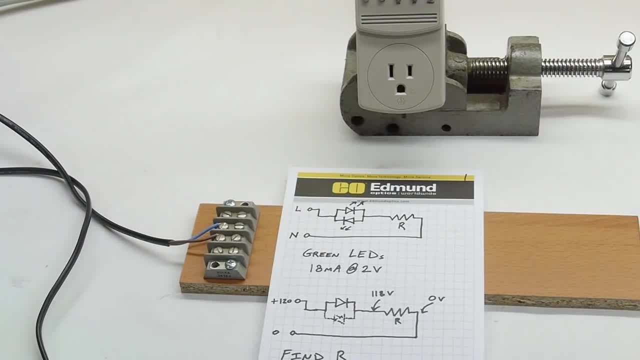 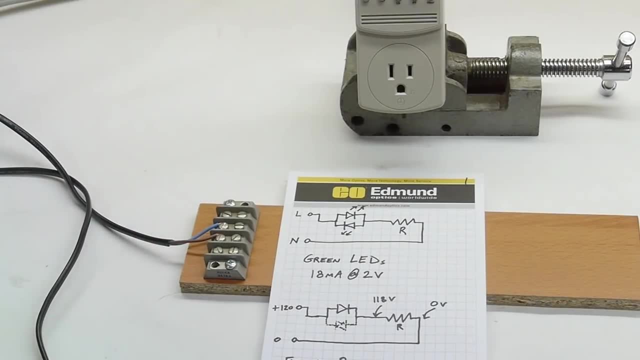 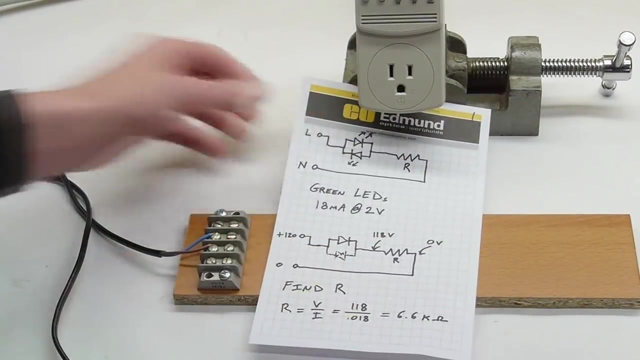 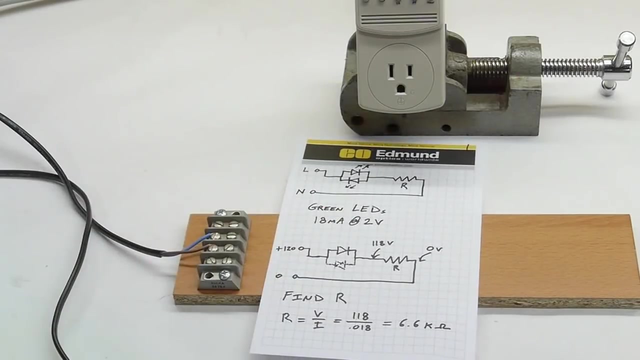 So what we can do to keep that from happening is to put a big fat resistor between the LEDs and the loop formed by the power source. So how do we figure out what resistor value? We can do that by measuring the LED. I measured this cheapo green LED and it just came up to be about 18 milliamps at two volts. And I got that number just by connecting it to my power supply. 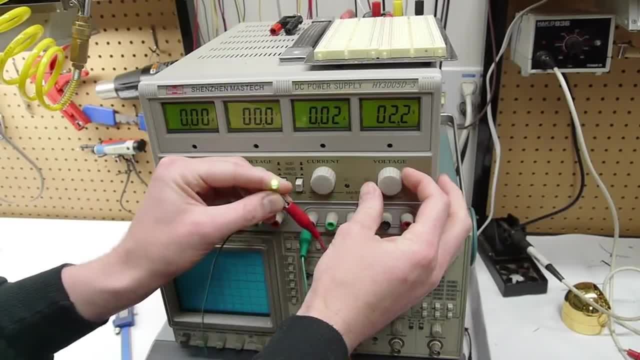 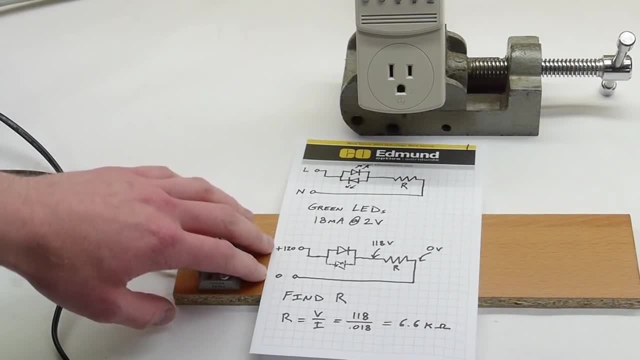 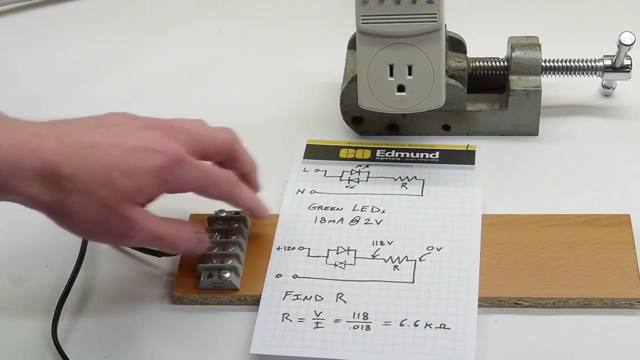 getting a really quick. you know rough reading. Okay, so if we know that the voltage across the line is 120 volts on average for one cycle, the current will flow out through the line, through the diode, through the resistor and back, And this whole thing reverses obviously when the AC goes into the other phase. So we'll just look at this one phase. 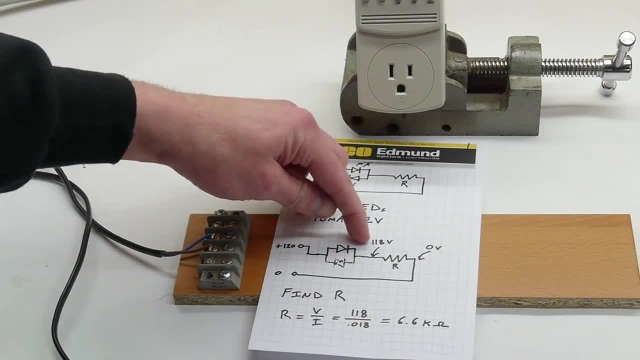 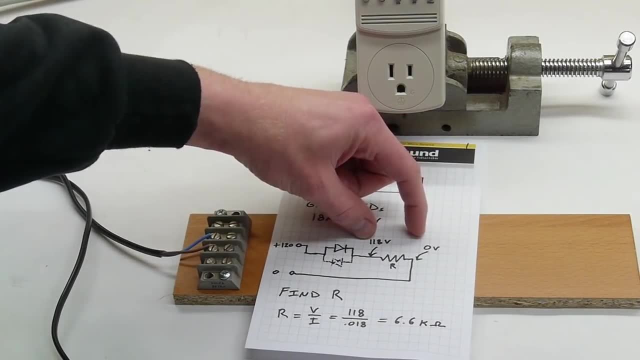 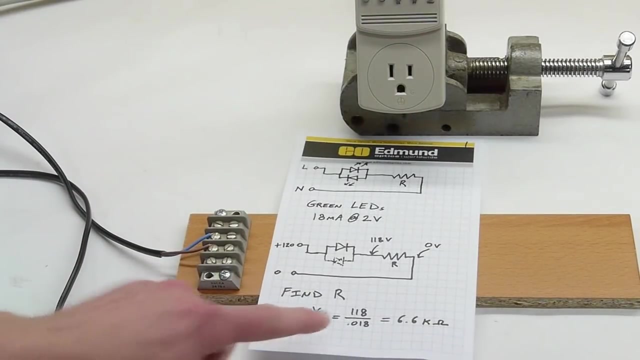 So we've got 120 volts here, 118 volts here because we know the diode is going to drop two volts at the proper current, And then the resistor has to drop 118 volts at the proper current. So then we just use Ohm's law: voltage over current, 118 volts over 18 milliamps- Remember to always enter the units in standard units, so amps, not milliamps- And we end up with 6.6 kilo ohms. 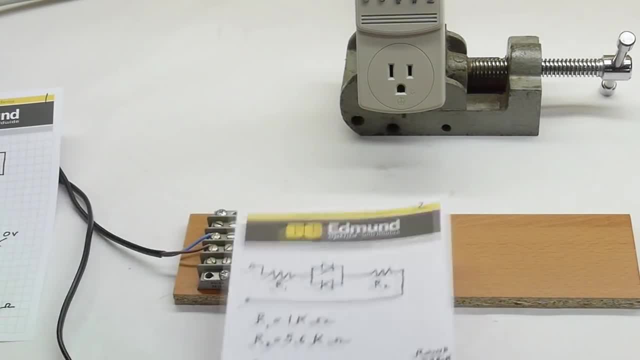 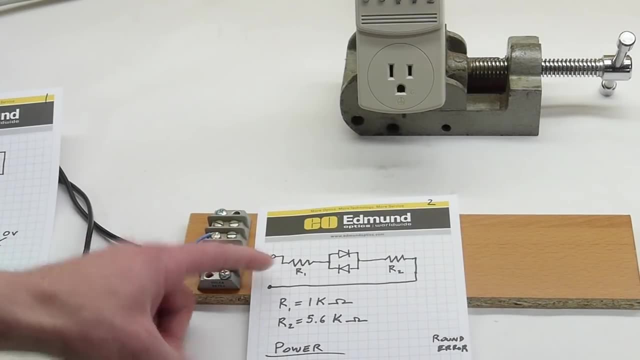 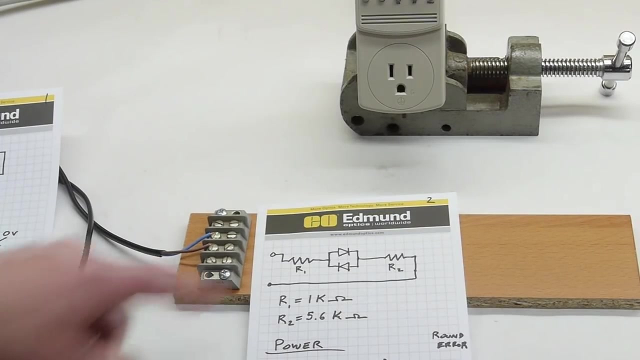 Okay, easy enough. Now what I'm going to do is just change that up just a little bit, And this will become clearer later on. What I'm going to do is put 1k here and 5.6k here, And that may seem a little strange right now, But this will make sense later on. The LEDs don't really care whether the resistor is on the left side or the right side, So splitting the resistance stuff like that doesn't really change anything with the circuit. So here it is. 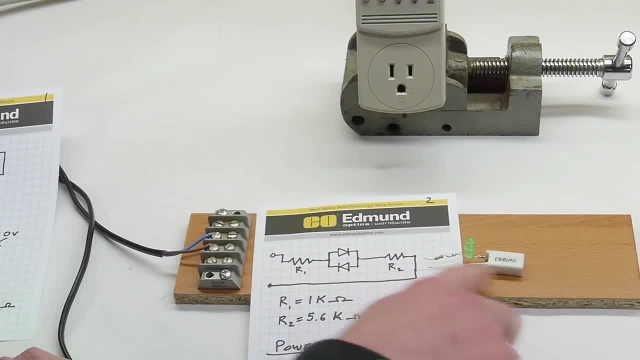 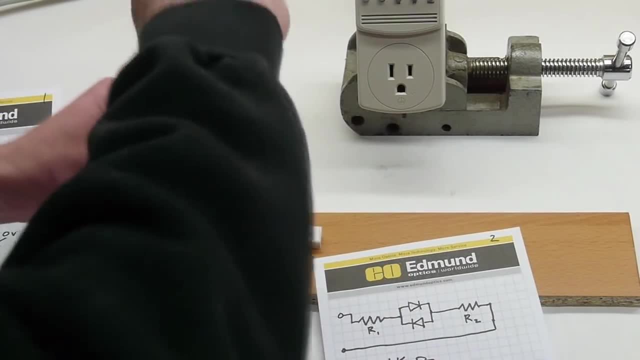 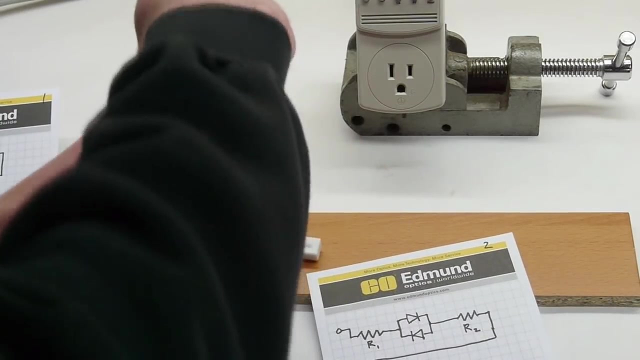 You can just see the small resistor, the two LEDs and this is a big resistor. Using a big resistor was necessary because this is going to dissipate some pretty serious power. I should also point out that, unless you're familiar with the hazards involved with you know AC line current, you probably would not want to try this one home. This is more of a demonstration. 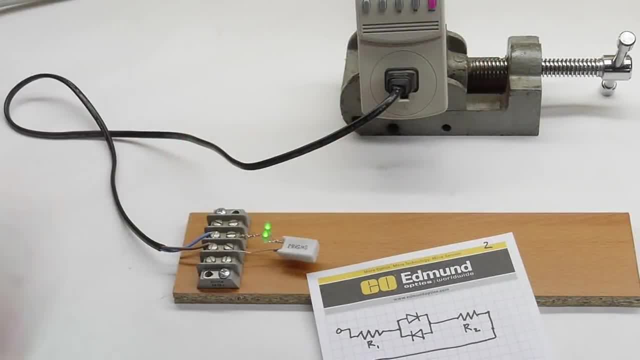 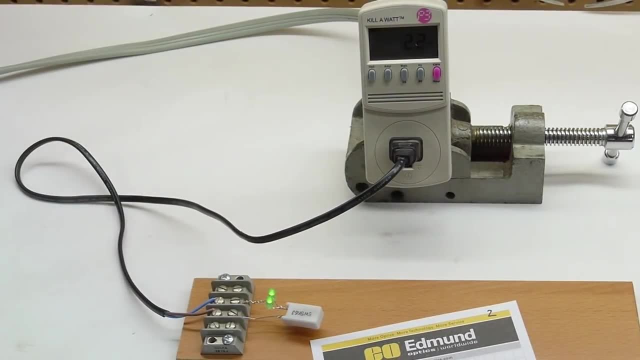 So I'm going to plug this in The LEDs, come on, And hopefully you can see: yeah, it's drawing about 2.2 watts according to this meter. So 2.2 watts for those two measly resistors, two measly LEDs, is not very good at all. 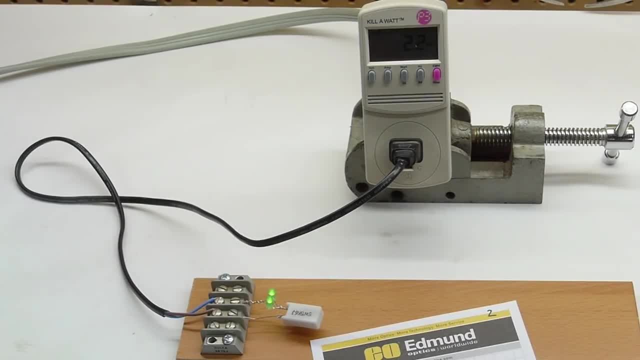 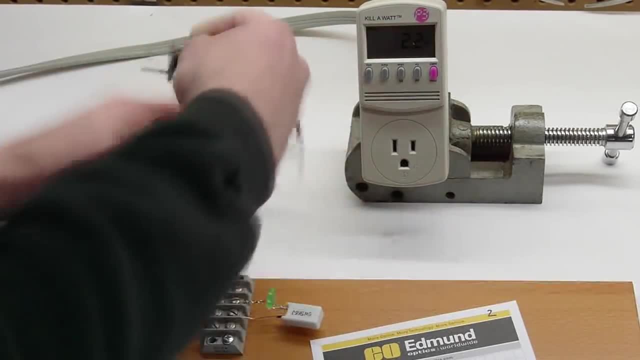 If you were an electrical engineer and you came up with this, the energy star people would not be very happy with you at all. So I'm going to unplug it And just after this, just after this five or 10 seconds of running, this resistor is. you know, it's not going to work. 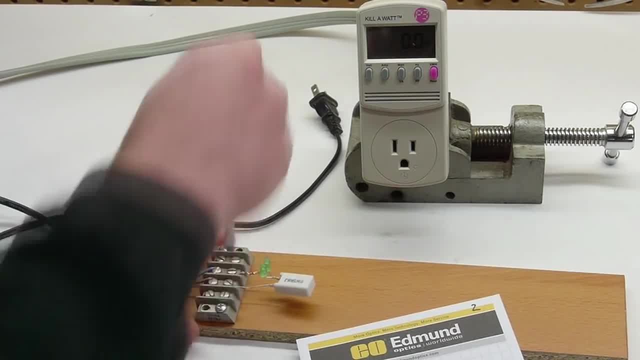 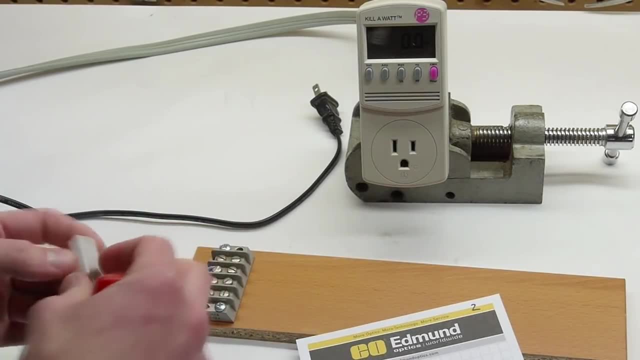 It's not burning hot, but pretty good and warm. And if this were left running for 10 minutes or something, that resistor might be too hot to even hold. It's a well, it's a five watt resistor. It would get pretty warm. 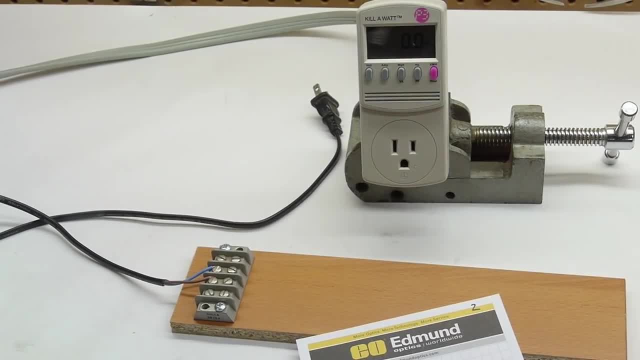 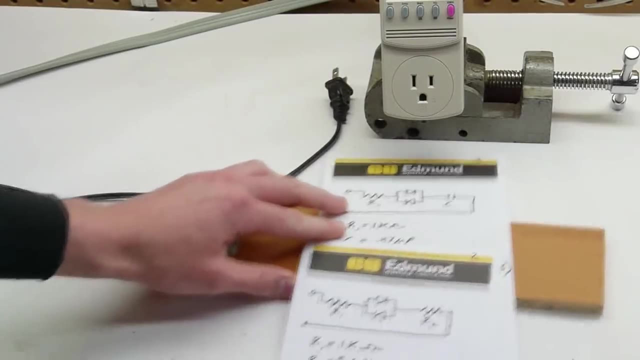 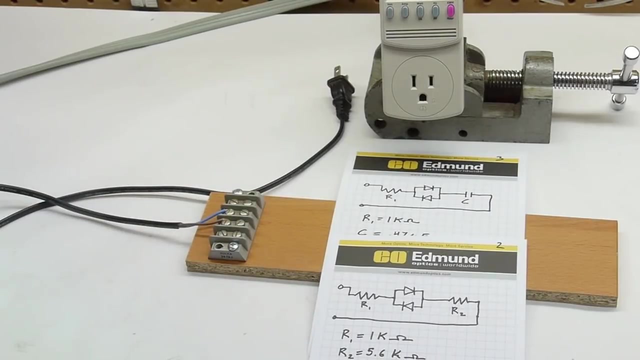 So we've got to come up with another design, And that design is this. So what I've done is replaced the resistor. This is the first design here. Hold on a sec. Basically, just replace R2 with a capacitor. So you might be thinking: well, what's that going to do? 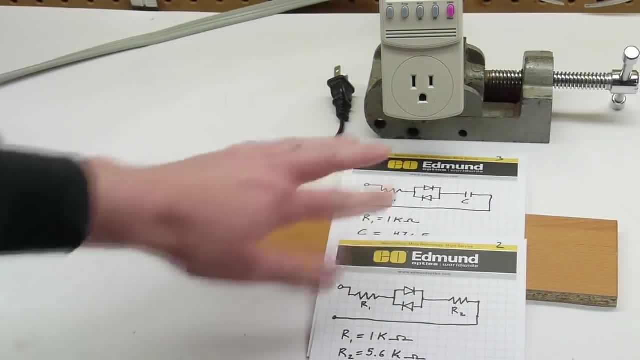 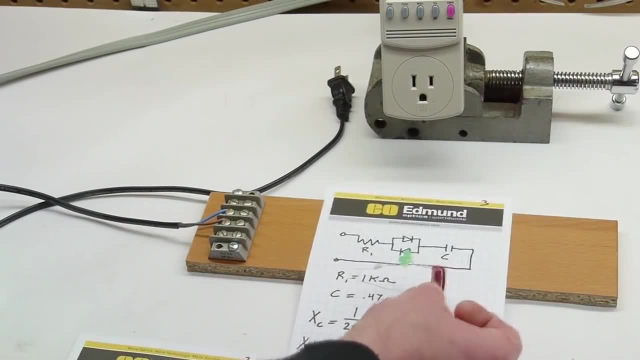 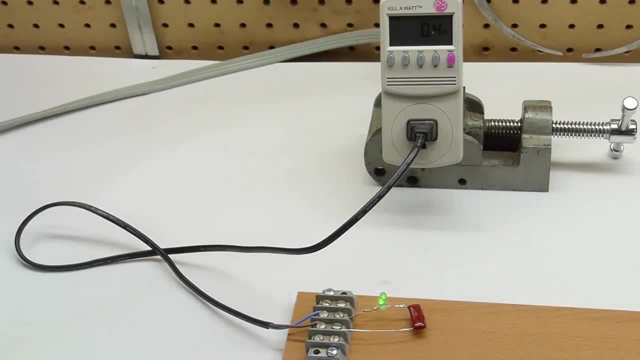 But notice the power meter: It's only drawing 0.4 watts instead of 2.2.. So our change- the change from a resistor to a capacitor- has actually made our circuit quite a bit more efficient. So let's take a look at why. 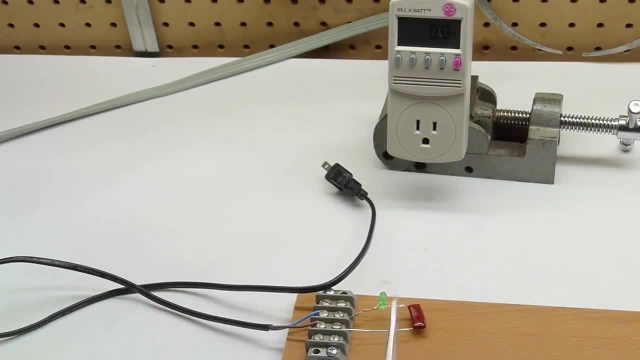 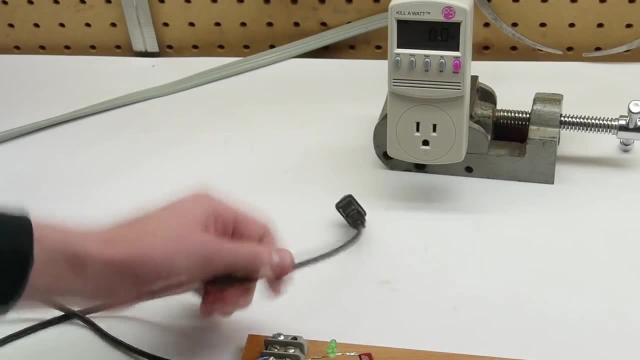 I'm going to unplug this and also discharge the capacitor. It had a little tiny pop. I don't know if you heard that or not, But you wouldn't want to if you did build this circuit. keep in mind that when you unplug. 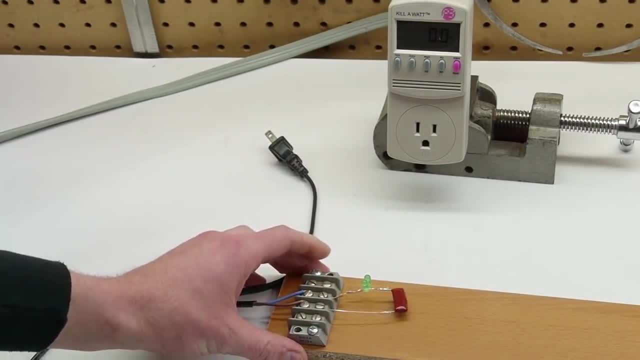 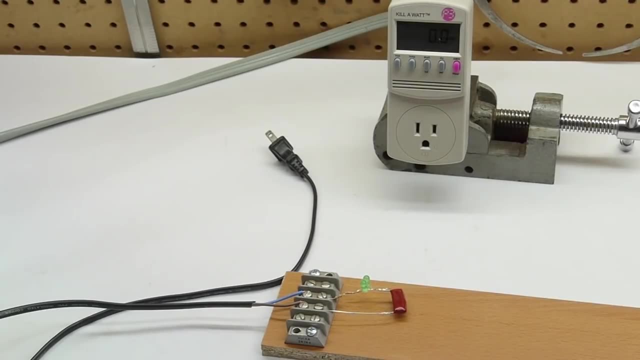 from the wall. it's going to discharge the capacitor wall here. that capacitor is going to store a charge and you know, just short it out like this, like i say you should probably be familiar with, with 120 volt safety if you're going to attempt. 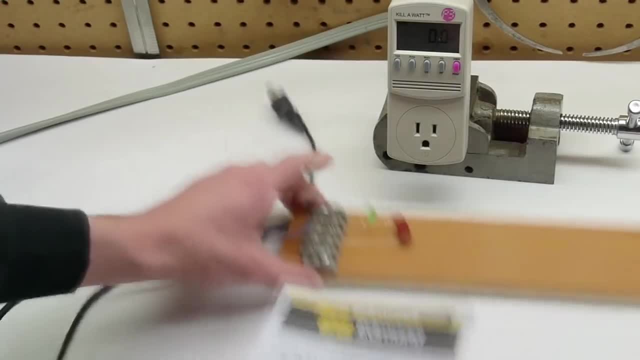 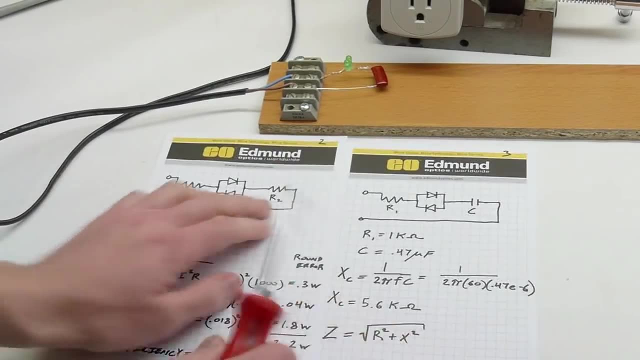 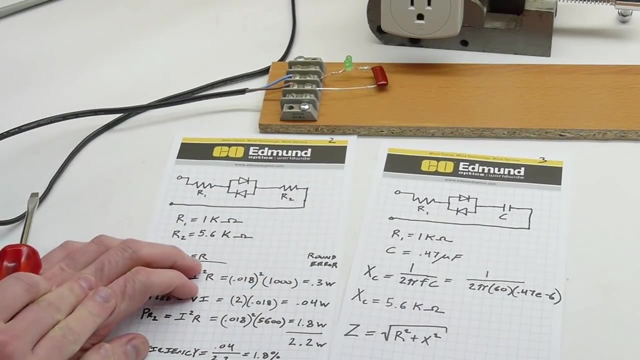 this one. so let's take a look at that schematic again. okay, so i said that the capacitor and the resistor in the in the first circuit are serving similar purposes. they're both restricting the amount of current that can flow through this circuit and this the units that we use to. 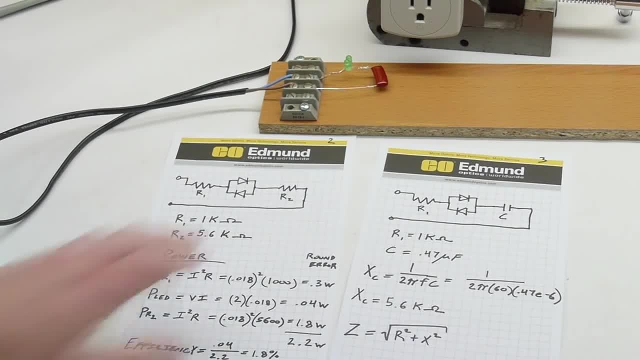 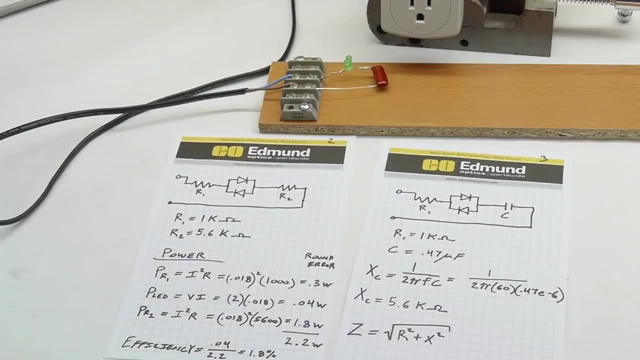 describe a restriction of current are ohms, so these both actually have a value that we can state in ohms. but why are capacitors not rated in ohms, like if you go to a electronics catalog and look down the list of capacitors, nothing is in there is going to say anything about ohms, so 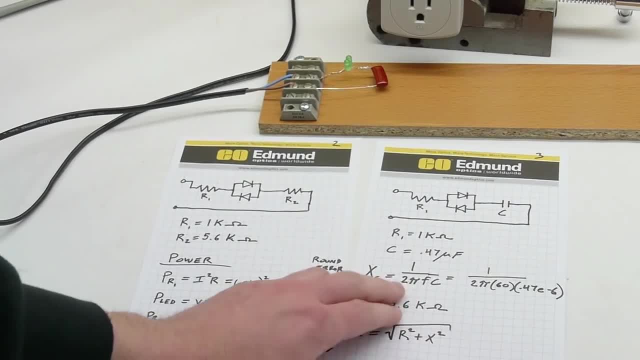 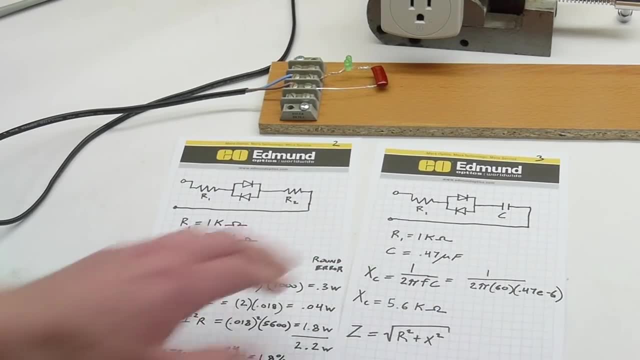 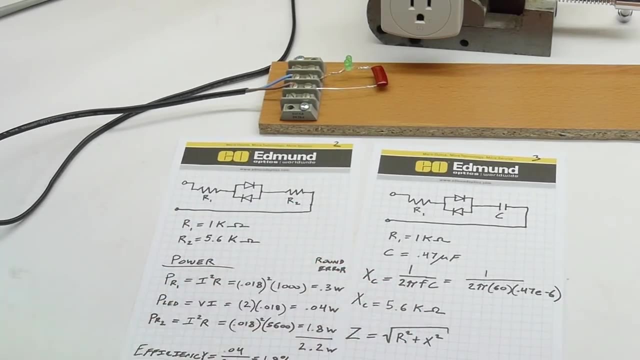 how do we do it? we use this formula right here: 1 over 2 pi, times the frequency in hertz, times the capacitance in farads. so this capacitor is 0.47 micro farads and the frequency is 60 hertz, because we i'm in the united states and all the line power is 60. 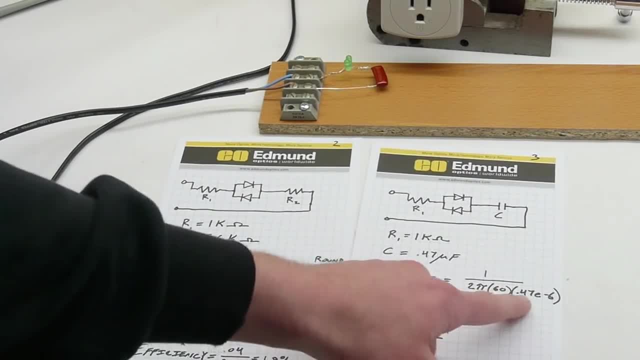 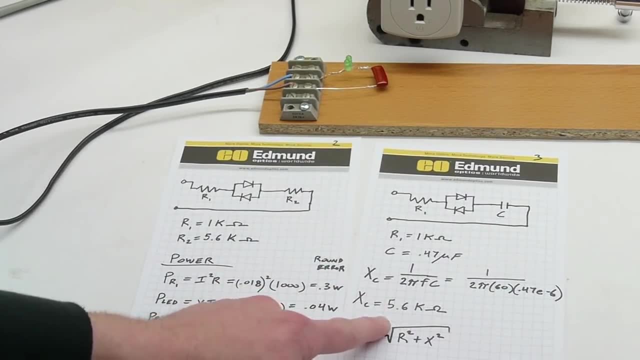 hertz here. so 1 over 2 pi, times 60, times 0.47, times 10 to the negative 6.. and if you calculate this all out you get 5.6 kilo ohms again. this is just like in the first circuit. they're almost exactly equivalent. 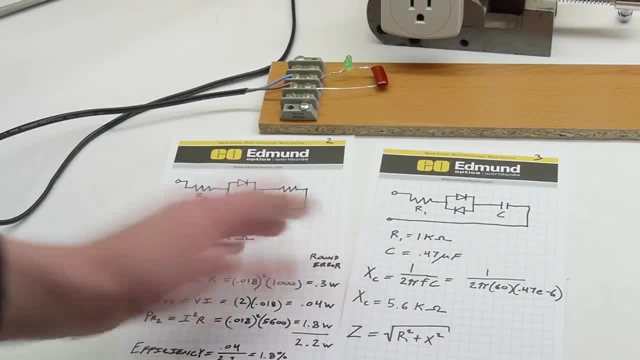 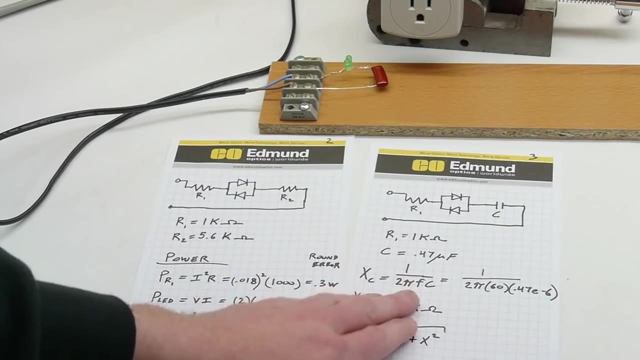 and so this, this value here, x, is called reactance, and reactance is basically a resistance to alternating current flow. so they're both, you know, in ohms. this is the same ohm value as the resistor. the difference is that the reactance depends on the frequency. 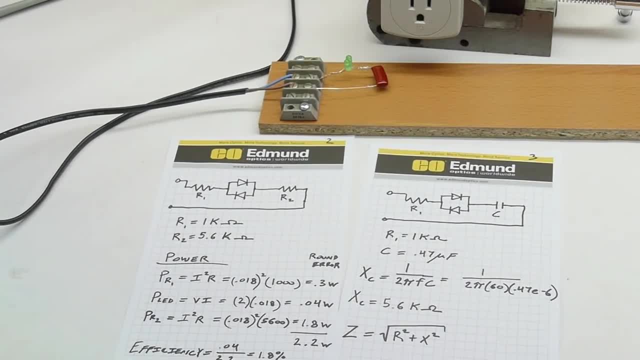 so the reason they don't print capacitors with ohm values in a catalog kind of circuit you're going to put it in. So if we were using this in Europe, where the power is 50 hertz, the Ohm value would be slightly different because the frequency is different. So what's? 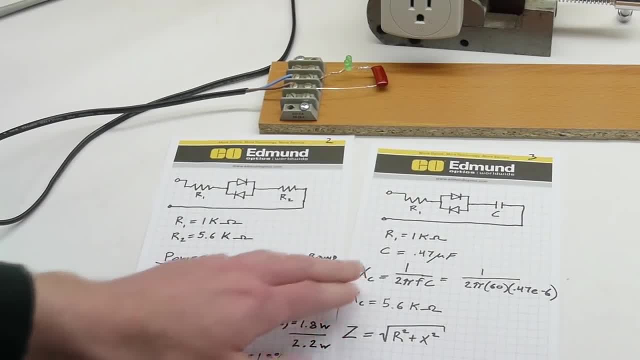 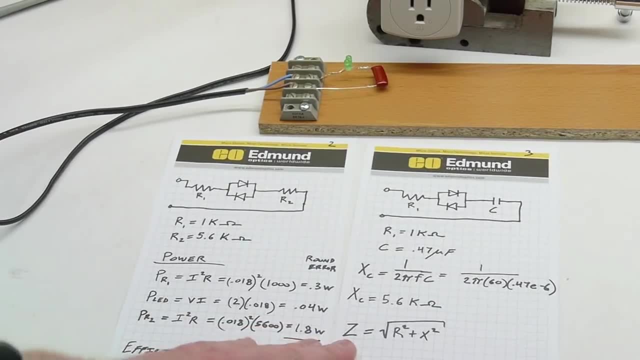 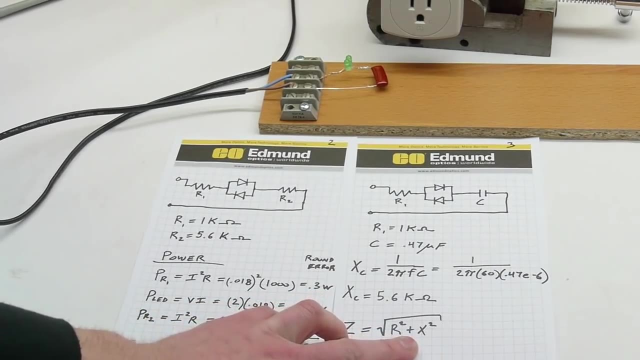 impedance. Impedance is the combination of reactants and resistance. Unfortunately, we can't just add them together. Impedance, which is represented by z, is equal to the square root of the resistance squared plus the reactants squared, And you geometry guys out there will. 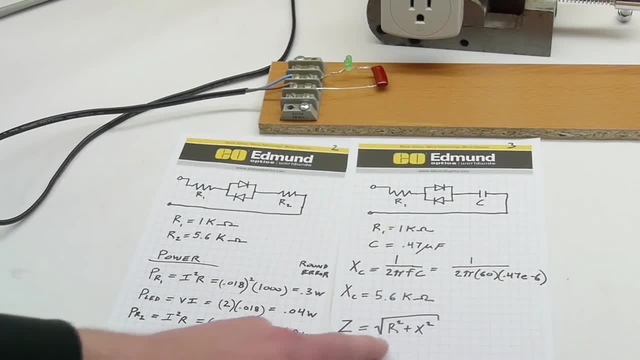 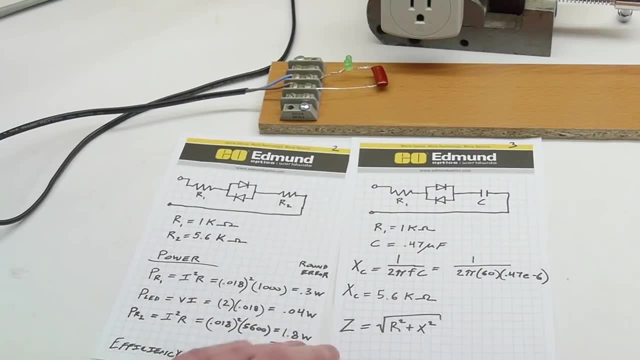 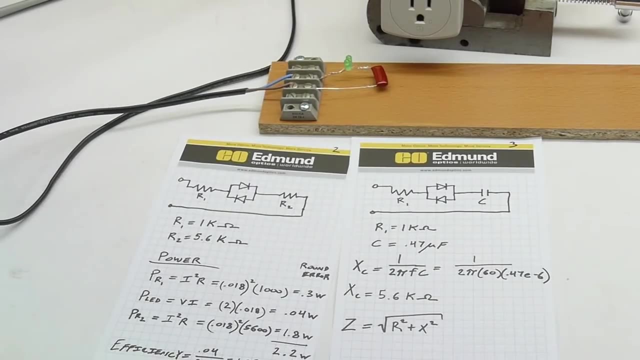 see that this is how to calculate the length of a hypotenuse, knowing the leg lengths of a triangle. So we'll get into this later, but just for now I just wanted to show you where impedance comes from. Impedance is just the combination of the pure DC resistance and the AC resistance known 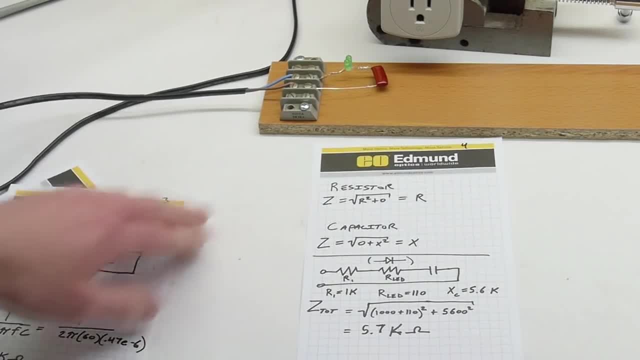 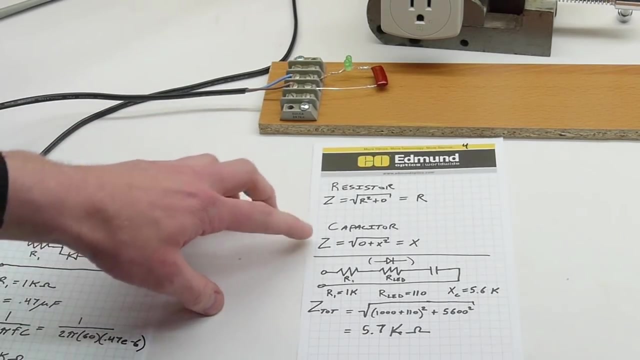 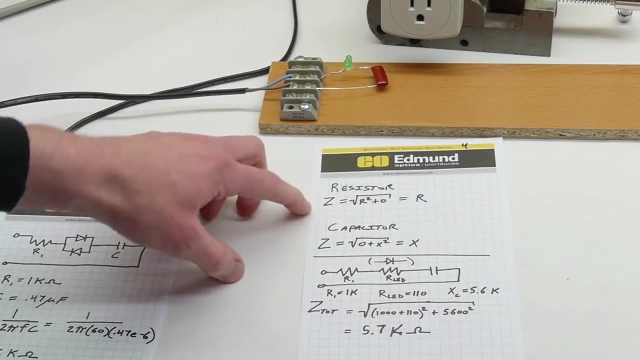 as reactants. So the impedance of a resistor, z, equals the square root of r squared plus zero, because a resistor doesn't have any reactants. A resistor has the same resistance at all frequencies if it's perfect. A capacitor has no resistance if it's perfect and it has reactants. So the impedance of a pure resistor is just. 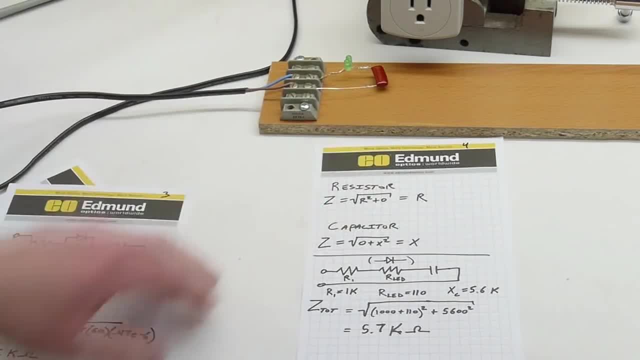 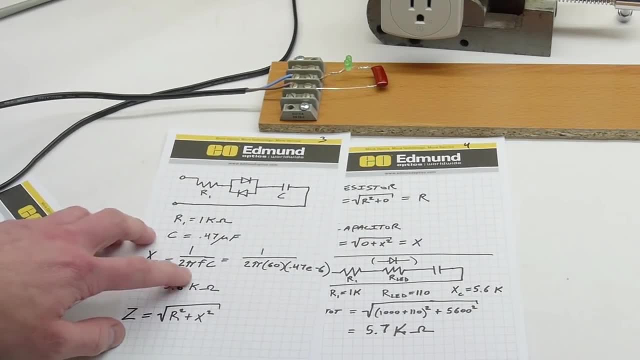 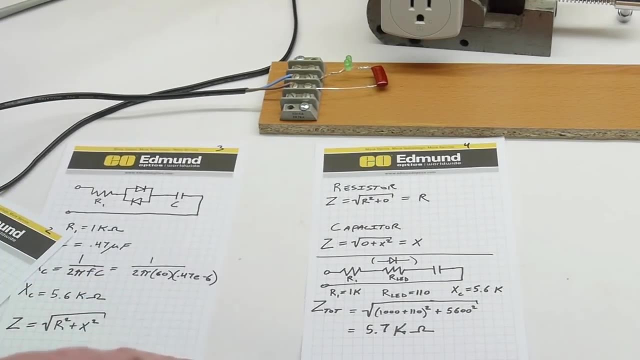 the resistance and the impedance of a capacitor is just the reactants And we had the formula here for the reactants of a capacitor: A capacitor is just one over two pi, the frequency times, the capacitance. So I'm just going to show you that you can't. let's say we wanted to know the entire amount. 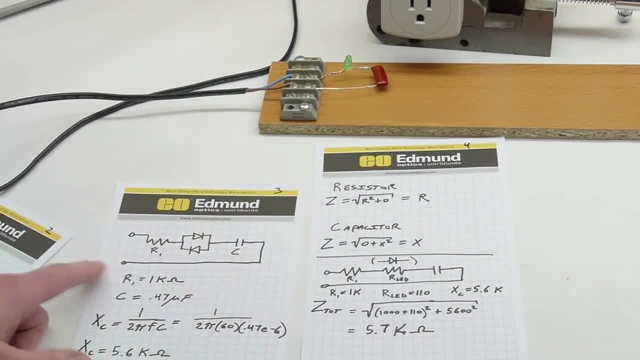 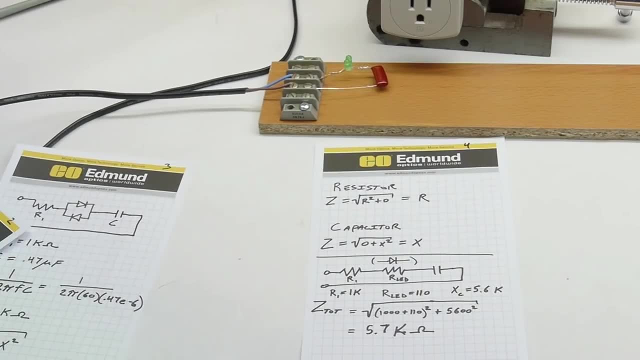 of impedance for our whole circuit here. What's the impedance for this whole thing? We're going to make a really nasty assumption here. We're going to assume that the LED actually behaves like a resistance, which of course it doesn't, But in this case it's not going. 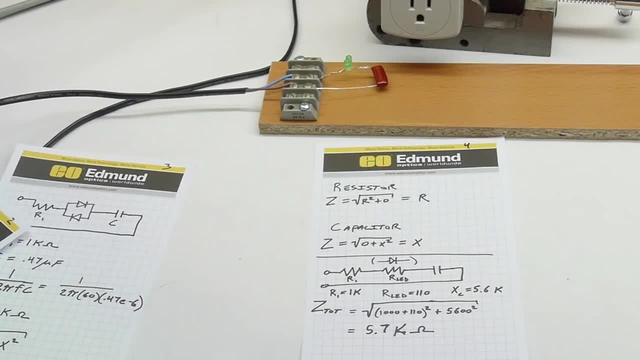 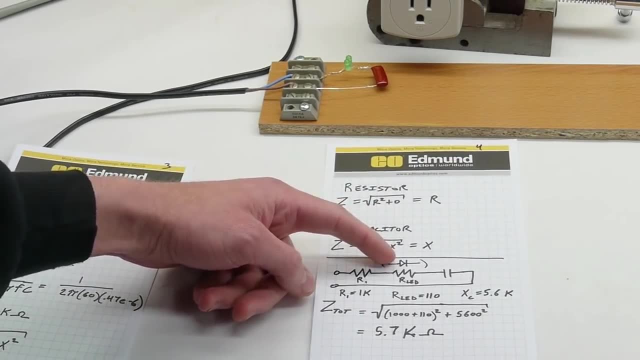 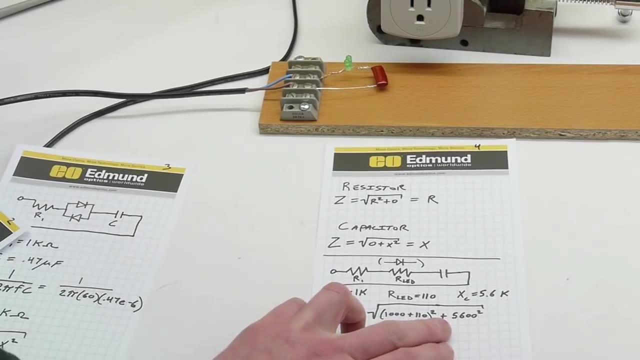 to make much difference because it's such a small part of the circuit. So here's the z total for our whole. we're going to approximate the resistor with a 110 ohm resistor. So we've got 1k plus 110 squared plus 5600 squared, and take the square. 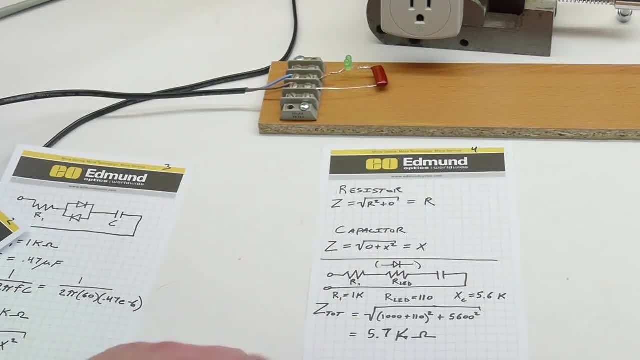 root of that. So the entire impedance for the whole circuit is 5.7 kilo ohms. So basically, impedance is just a resistance that depends on frequency. That's really all it is, And so with a capacitor at higher frequencies it will have a lower impedance and a higher 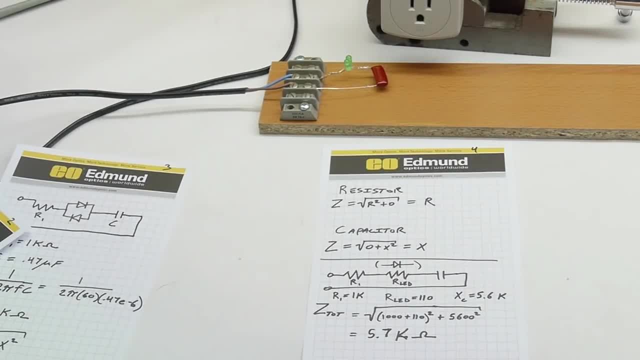 impedance at lower frequencies. So think what would happen if you took a capacitor and just put it across a power supply. Once the capacitor charges up, no current flows, because that capacitor is infinite resistance at DC currents. Let me just draw this out here. 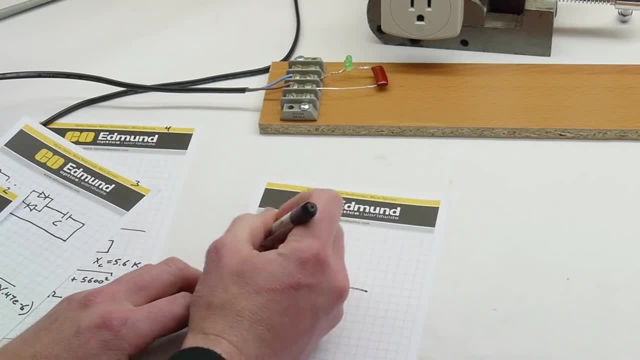 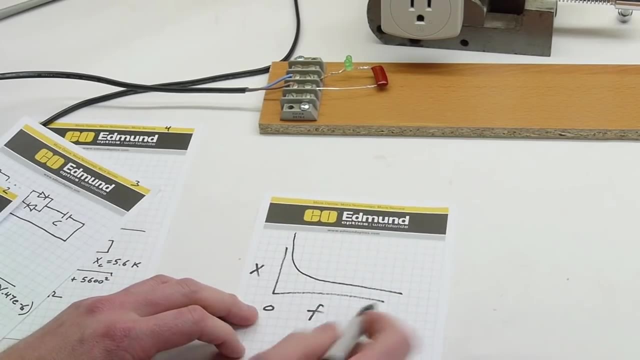 For a capacitor. this is reactance and this is frequency. When the frequency is low, it's zero. basically, the reactance is infinite. At the high frequencies, the reactance becomes a very low value and this has a 1 over f relationship. 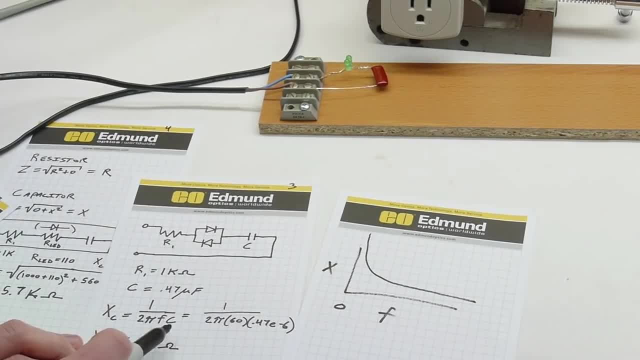 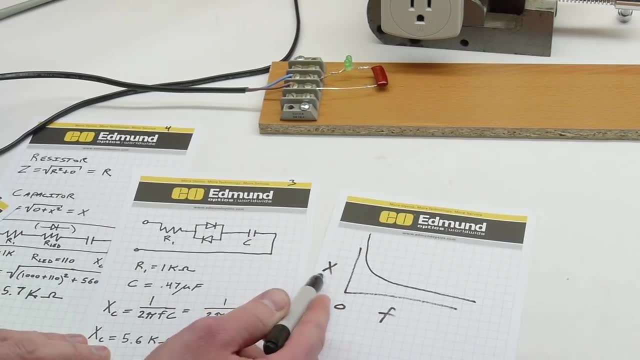 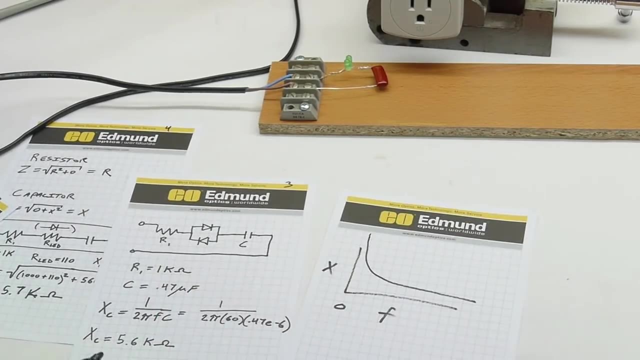 because of the formula We had 1 over 2 pi fc. So you can see that for any capacitor at zero the reactance and resulting impedance is infinite, And at infinitely high frequencies the reactance is zero. So for infinitely high frequencies a capacitor is like a short. 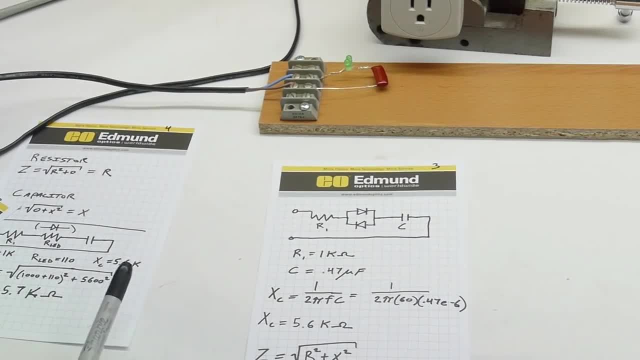 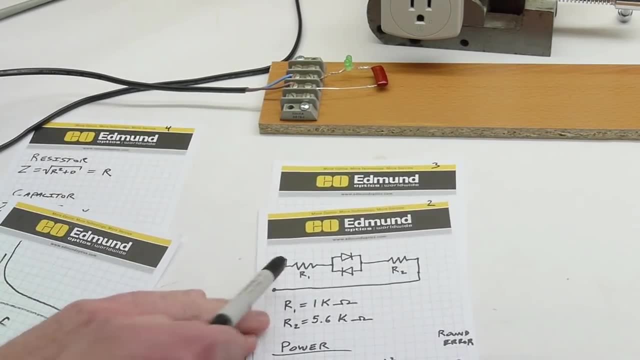 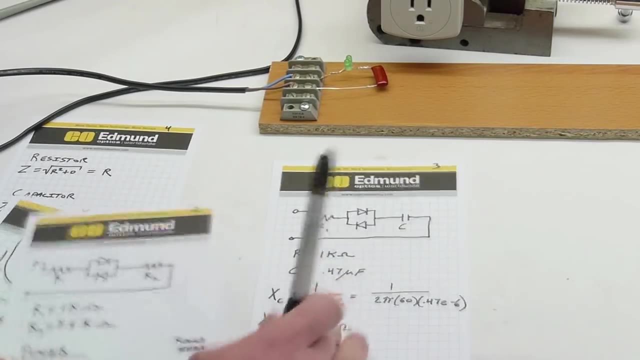 Sometimes the water analogy is helpful. So think of electrical current, like water flowing through a pipe In the case of a resistor in our circuit. here The electricity flows, The water flows through here and is restricted. The flow is restricted by these resistors. 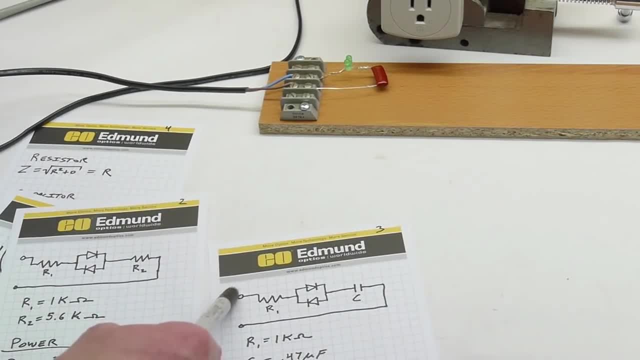 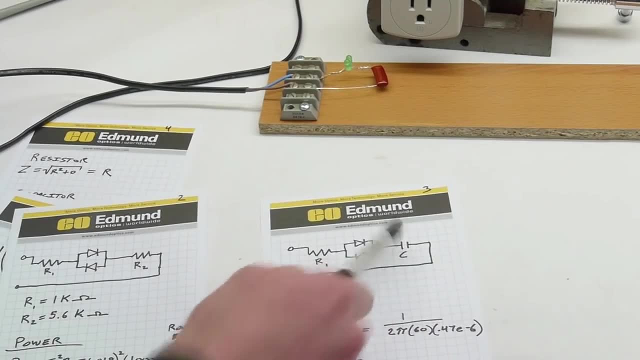 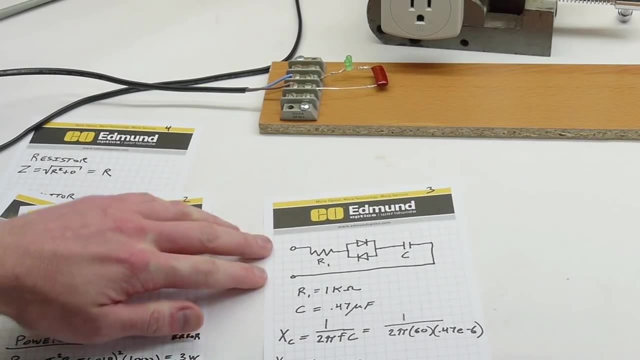 But in the case of the capacitor, the water or electricity flows into here and the capacitor acts like a bucket. So the water flows into the bucket and it fills up the bucket And once the bucket is full, nothing continues to flow. The circuit basically stops. 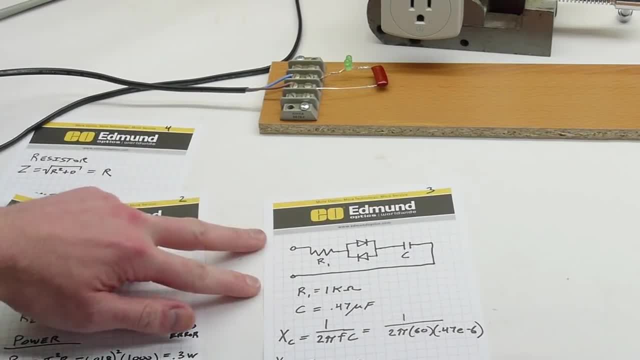 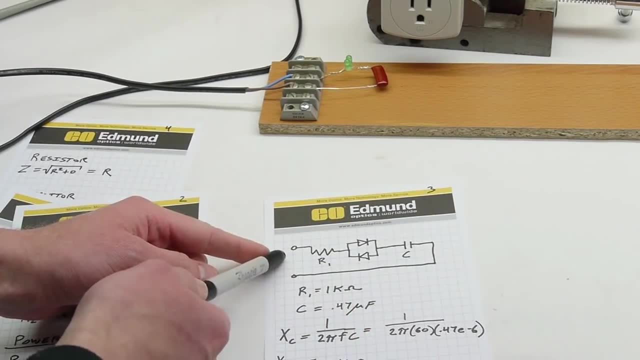 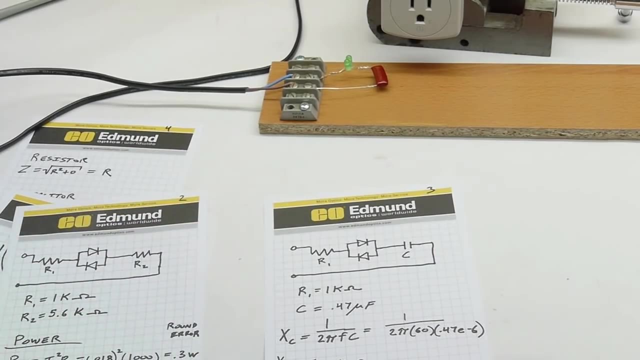 But in an AC circuit the voltage flips, in our case 60 times a second. So when the voltage flips polarity, the bucket dumps its contents back through the circuit and makes these LEDs light up. So you might be wondering: how does our circuit become more energy efficient? 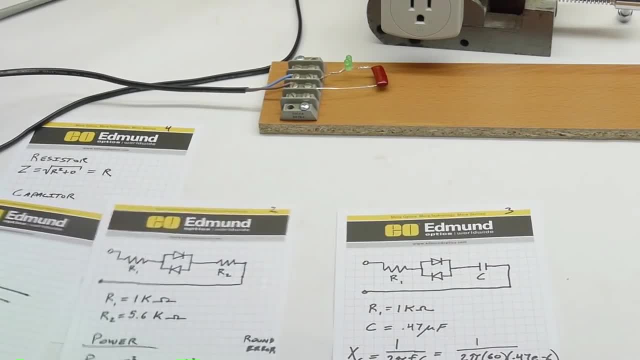 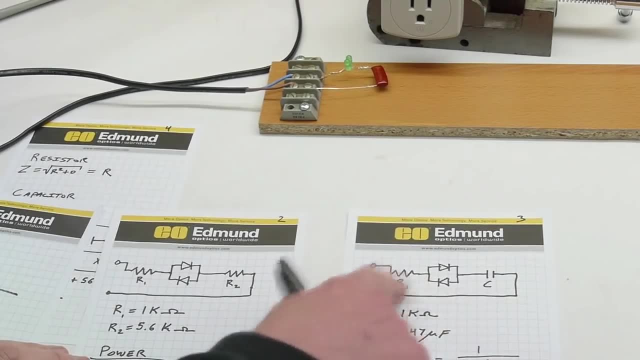 It has the same impedance. We said that we showed that these circuits are almost equivalent. We had 5.6k for this resistor, 5.6k for this capacitor. This is the same. This is the same. How come the power meter only read 2.2 watts? 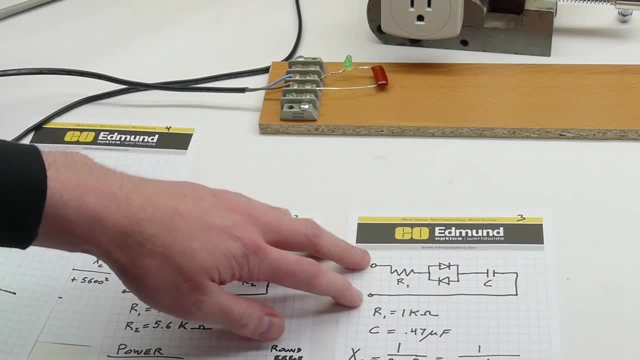 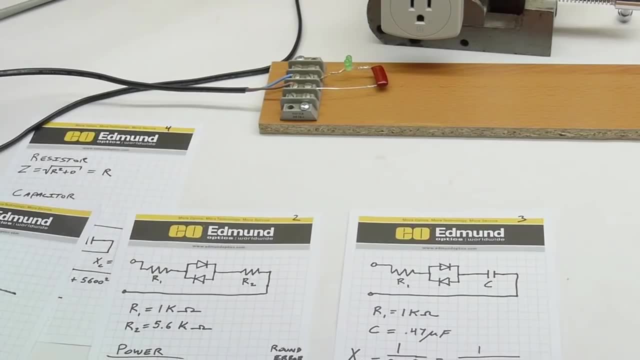 For this capacitor For this case, And only 0.4 watts for this case. We're going to talk about that next time in the exciting conclusion to our series on impedance here, where we're going to talk about power factor, volt amps and watts. 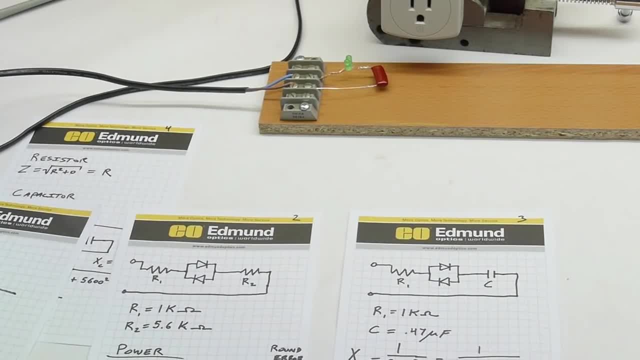 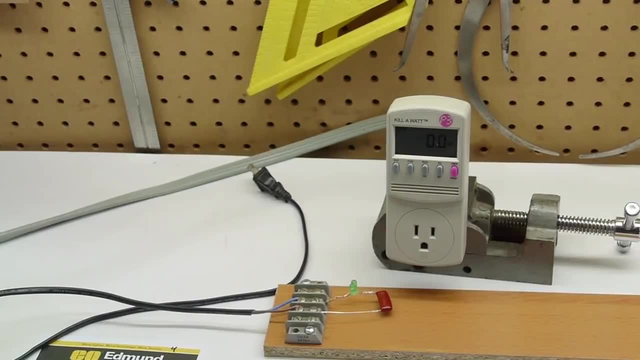 If you've ever wondered about those things, I'm going to talk about those next. You can actually use these cool little power meters to measure power factor, volt, amps and such. Okay, I hope that was helpful. Stay tuned and subscribe For future electrical tutorials, and feel free to post comments about what topics you'd like. 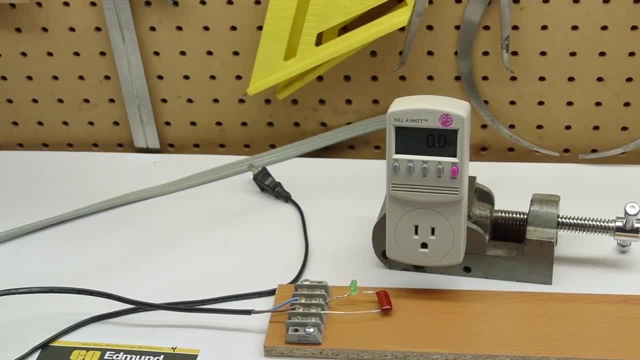 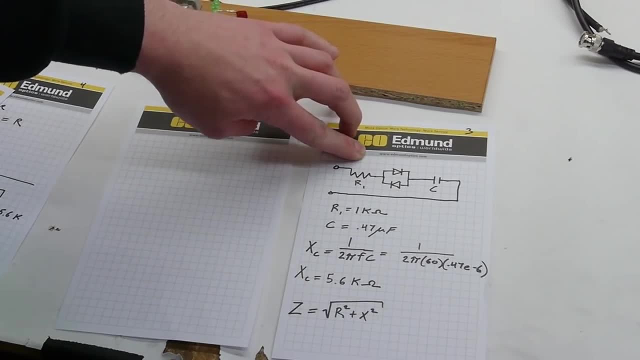 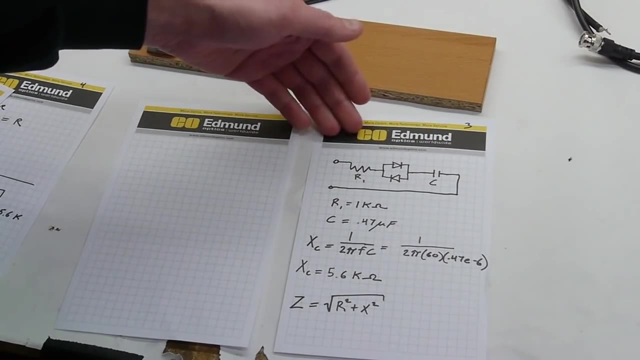 to see. Okay, see you next time. bye, Postscript. So you might be wondering why I left this resistor in with the capacitor circuit. I said that we could size a capacitor such that it would replace almost any impedance that we want in this circuit. 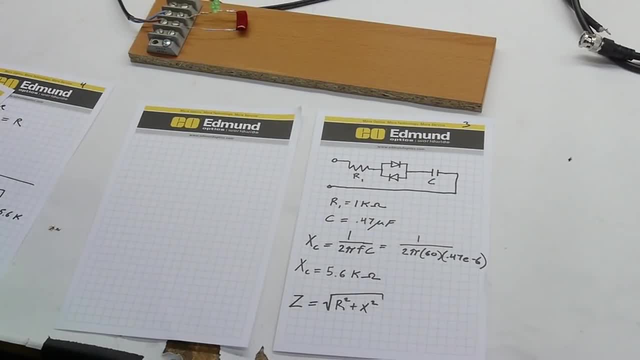 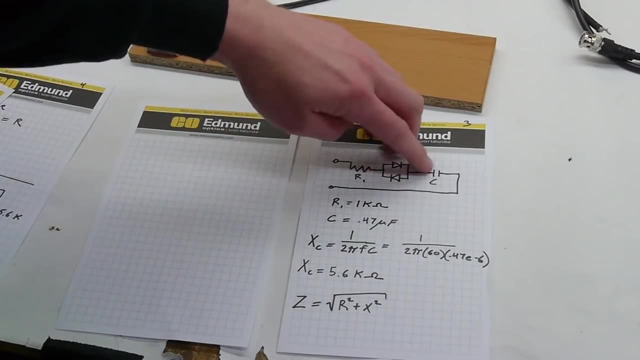 So why did I bother leaving this resistor in? It's actually more of a practical matter. I mean, in a perfect world we definitely could build this circuit without any resistance and make it purely capacitive. use just a capacitor to limit the current. 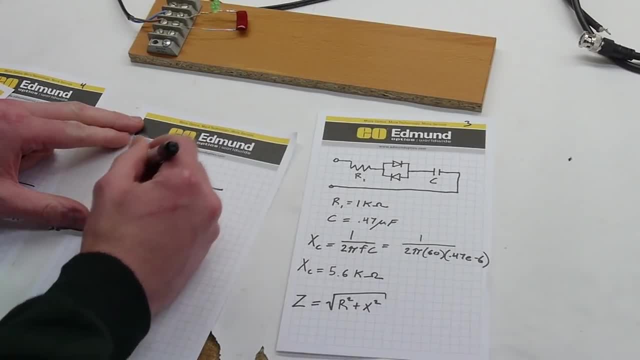 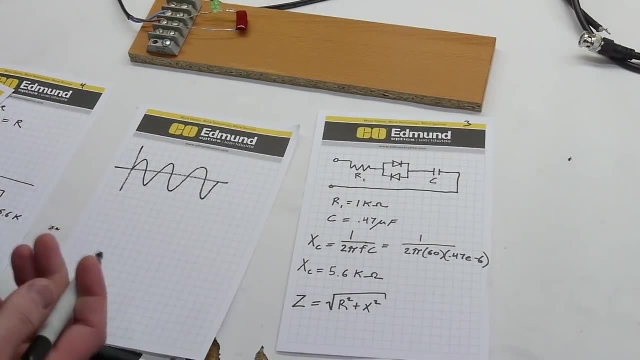 But here's the problem. In AC current, you know, we have a cycle that looks like this And at some point we have to build our circuit and then plug it into the wall. So if we happen- and this is just running constantly- 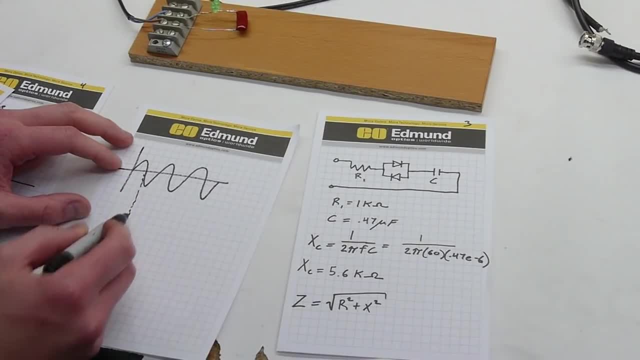 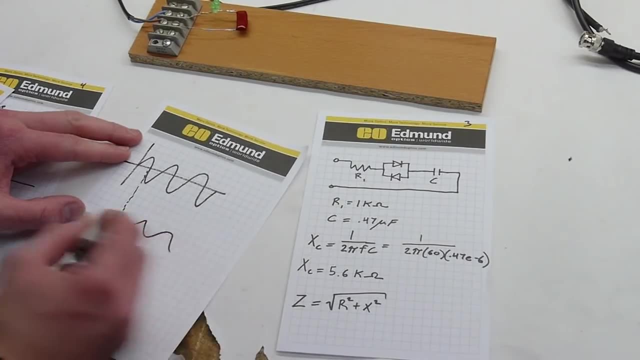 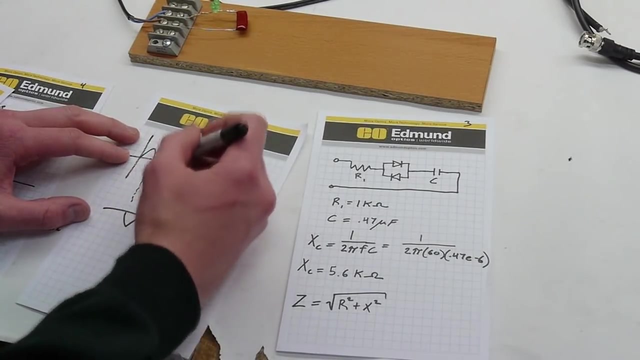 So if we happen to plug in our circuit right at this point in time, Everything would be great. The circuit would see a wave. that was nice and you know, starting at zero and flowing up and down normally. But what happens if we decided to plug in our circuit here? 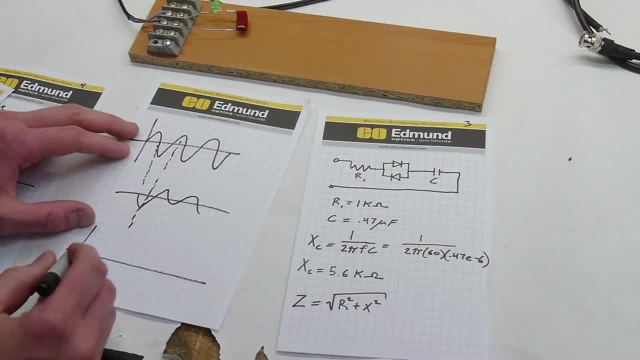 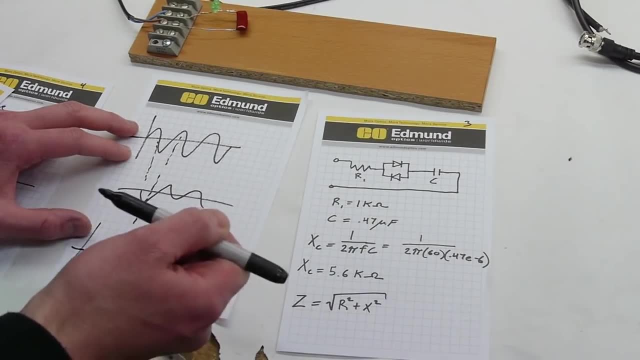 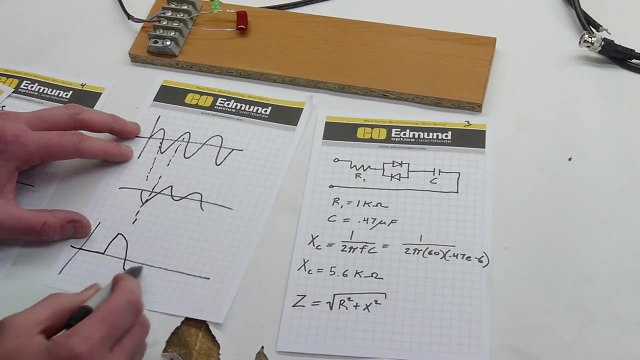 That wouldn't be so good. So then you know, if zero is here, our circuit would see something like this: Voltage would be zero, and then suddenly we put the plug into the outlet and suddenly we get a nice circuit, A nice sharp transition right up like this and then a nice smooth sine wave. 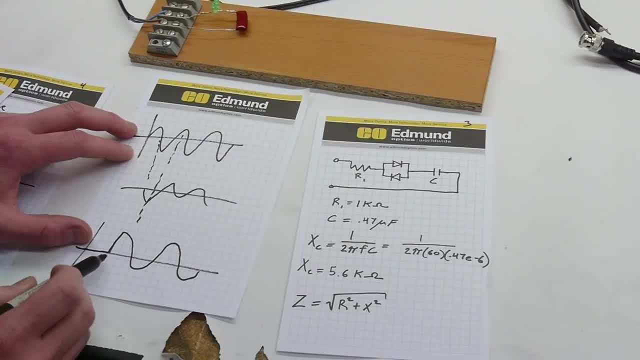 Now, this sharp edge right here is not 60 hertz. It's actually composed of a bunch of frequencies, many of which are higher than 60 hertz. So our capacitor has a much lower impedance during this very sharp spike, this very sharp. 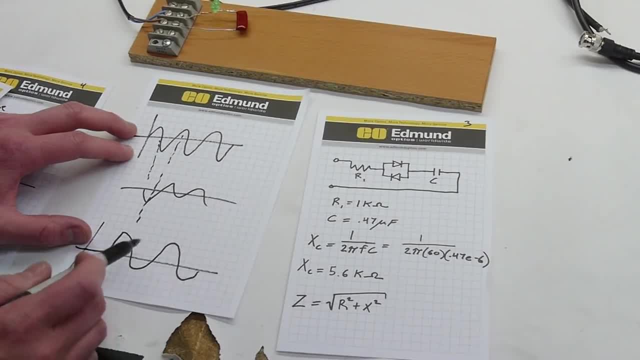 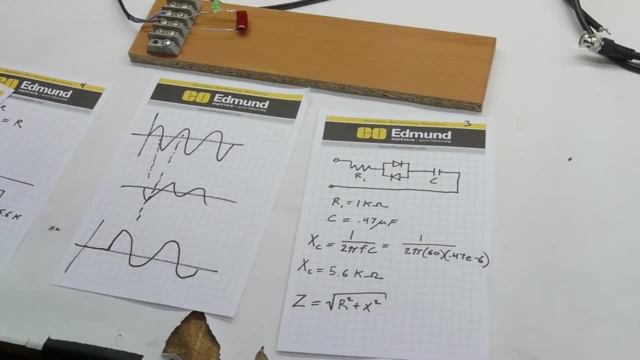 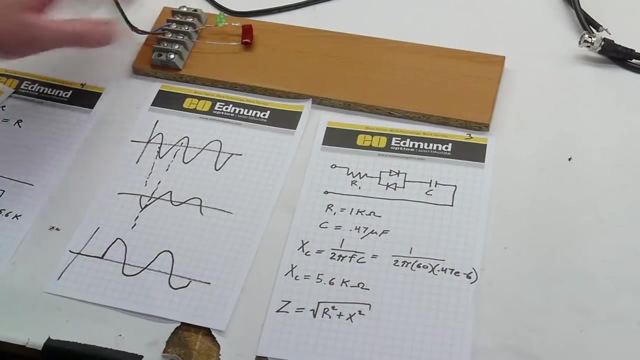 voltage transition And that would cause too much current to flow, It would cause the LED to die. So I tried it, You know. obviously I wanted to find out what would happen myself. So I built the circuit, you know, just like you see here, without the resistor, and plugged. 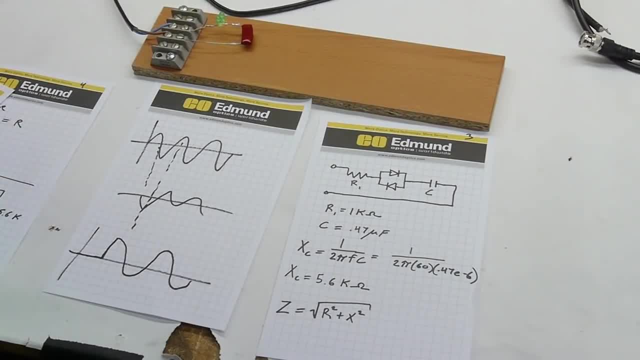 it in And after about 10 cycles of me plugging and unplugging it, the LED was just about toasted. It was still light, but kind of dimly. It wasn't doing very well. So during this really short time, this is probably only going to last about a millisecond. 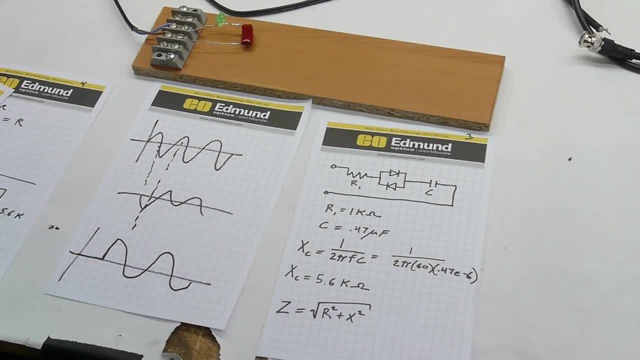 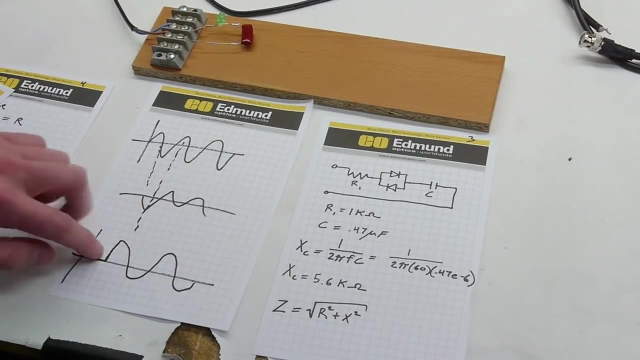 there will be much higher current flowing through the LED. So this limits the so-called inrush current And it's purely a practical matter, just because you know you can't plug in your circuit at the zero crosspoint every time. You have to anticipate this sudden surge.